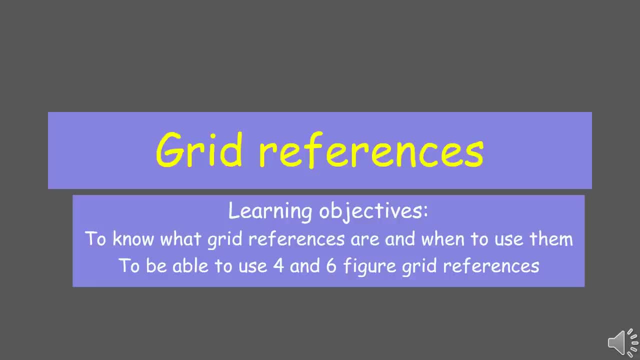 Hello everyone. In this video we're going to be looking at grid references. By the end of the video, I would like everybody to know what grid references are and when to use them, and also to be able to use four- and six-figure grid references. 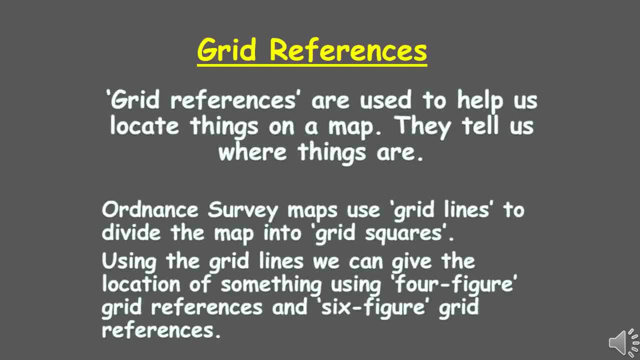 The basic purpose of a grid reference is to locate things on a map. They tell us where something is On the Ordnance Survey maps. we use these imaginary lines, which we call grid lines, and they divide the map into grid squares. 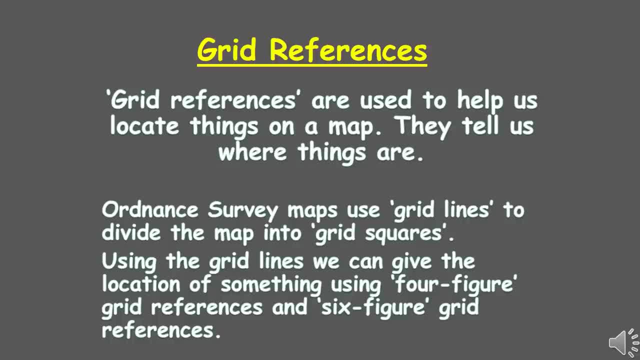 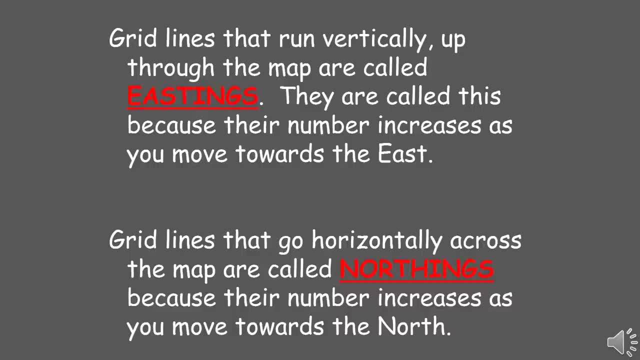 These lines can give us a location of something, either using a four-figure reference or a six-figure reference. There are two different types of grid lines: Some that run vertically upwards. These we call eastings, because their number increases as you move towards the east. 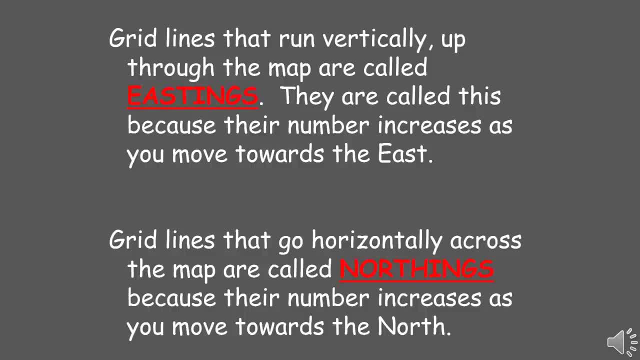 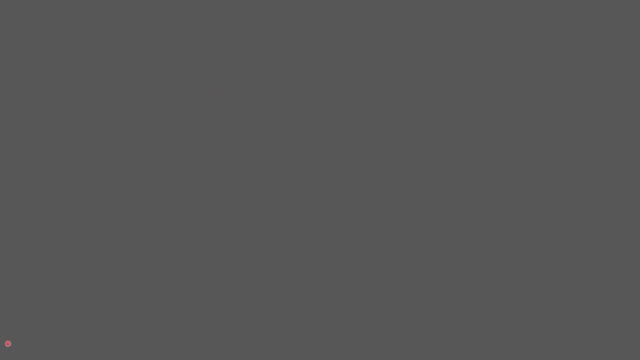 And the second type we call northings. These are horizontal lines, and that's because their number increases as you move towards the north. Now let us examine exactly how these grid references work. What I'm adding now is I'm adding the eastings, So these are the vertical lines. 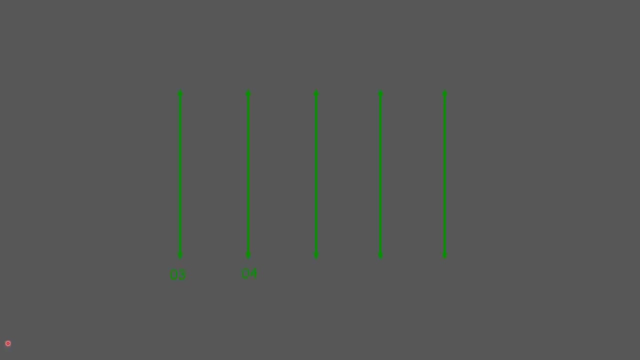 And you can see it that I'm giving a four-figure reference. I'm also giving them a number. They have to be two numbers to be able to fit in with the proper way of working out grid references. In this case I'm running from 0-3 all the way up to 0-7.. 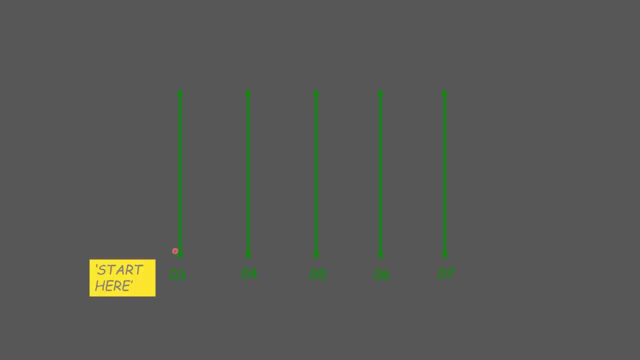 We start from the left-hand side over here. So 0-3 would be the first one that we would read, And we read going alongwards. Now I'm going to be adding in the northings: These are the horizontal lines that we read second: 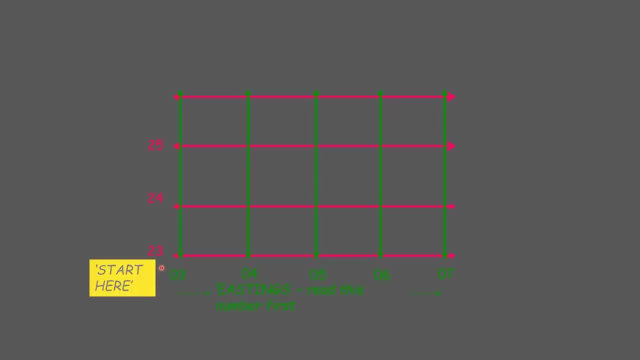 In this case the numbers don't change. They're going to stay the same. They don't have to be the same or follow the same sequence. So I'm going with 23,, 24,, 25, and 26,, just to make it a little bit different. 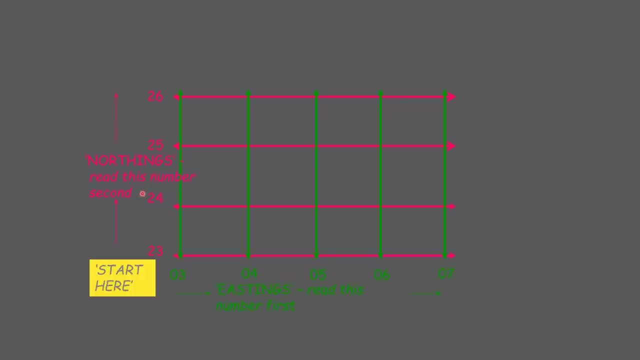 And we read the northings second. Now look at this yellow box. If we want to tell where this yellow box is on a grid, the first thing that we need to do is we need to read the eastings. We check 0-3,, no 0-4,, no 0-5.. 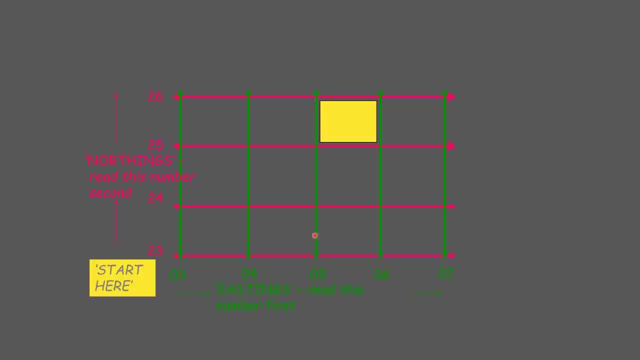 0-5 is the first line Or the first easting that comes into contact with this box, And then we work our way up: 2-3,, 2-4,. 2-5 is the first northing line that comes into contact with this box. 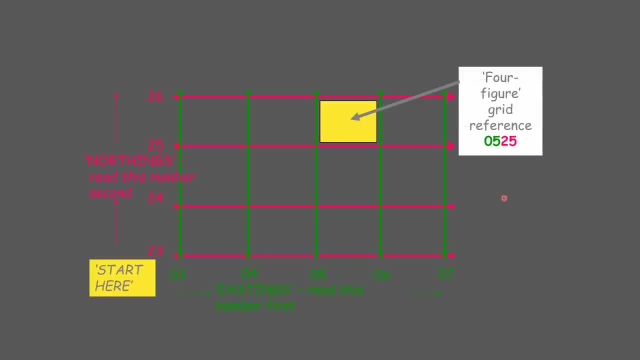 Therefore, this yellow box would be grid reference 0-5, 2-5.. However, this only tells us a large area. Now, on a map, this area could be very large in size. It could be a few kilometers squared. 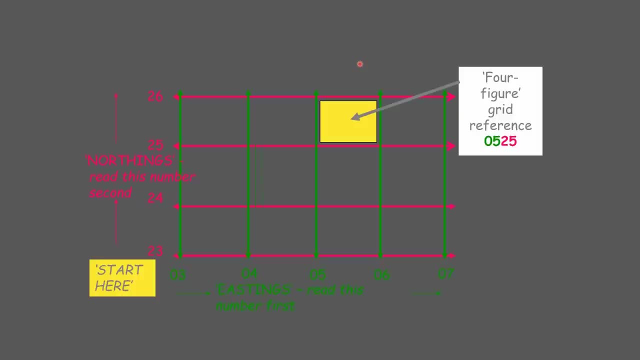 So if we want to be a little bit more precise, we have to break down each of these squares into subsections. As you can see, I'm adding them now. In reality, these on a map would not exist. You would not be able to see them. 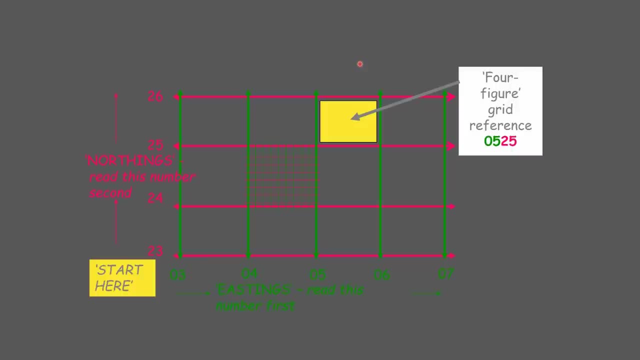 And therefore you'd have to mentally put them in there or at least use your ruler to work them out. What I've done is I've divided up the space between 0-4 and 0-5 eastings into 10 equal parts. 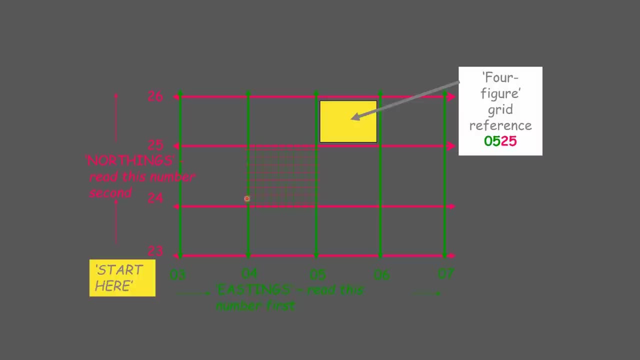 And I've divided up the space of the northings between 2-4 and 2-5, again in 10 equal parts, making a smaller grid reference over here. Now, if we want to find this more precise yellow square or say a feature or a symbol that's found in this area, 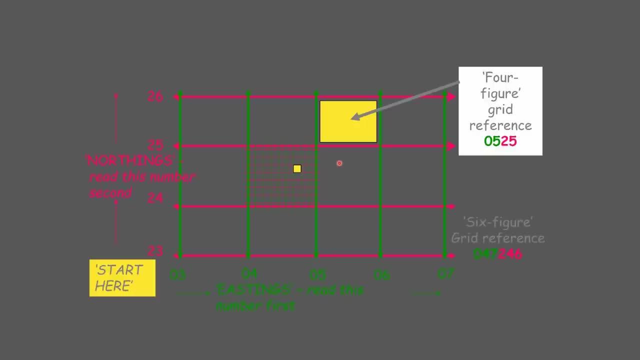 what we have to do is we have to ensure that we read it in exactly the same way. Firstly, we start by finding the integral. In this case it is 0-4,, 2-4.. Then, after the 0-4,, we have to work out which section inside this grid it is. 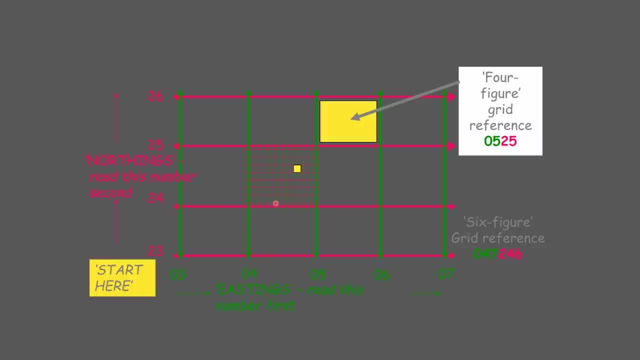 So it would be 0-4,, 1,, 2,, 3,, 4,, 5,, 6, 7.. There we go, 0-4, 7.. And then we work our way up: 2-4,, 1,, 2,, 3,, 4,, 5,, 6.. 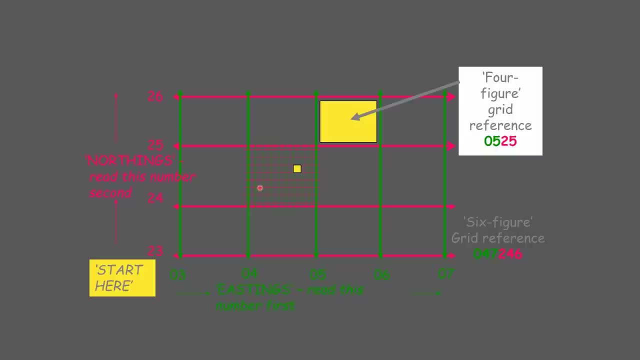 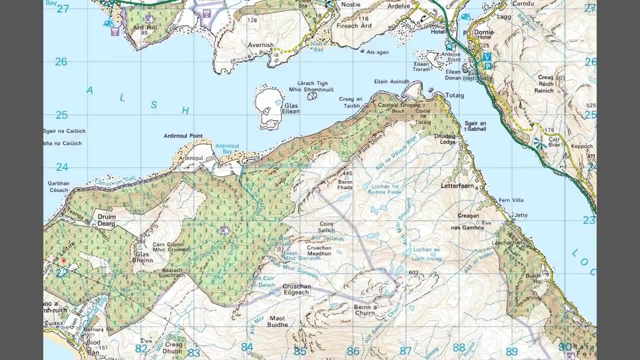 There we go. Actually, that's it. We should have started 1 from here, So it would be 0-7,, 2-4, 6 in this instance. This is now a proper ordnance survey map. The grids are not as clear to see. 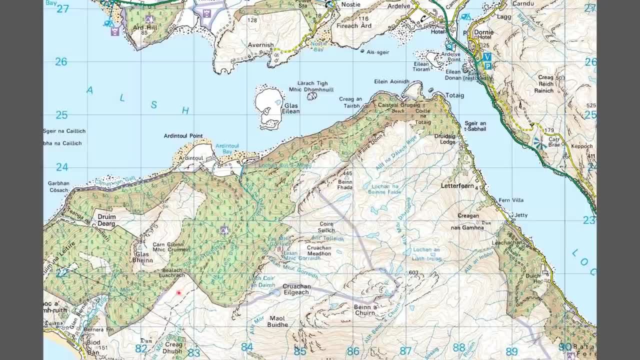 You can see these blue lines over here. These are the eastings. And then we go. these are the northings. We start over here from 82.. We start over here from 21.. Now let us presume we want to find the grid reference of this square. 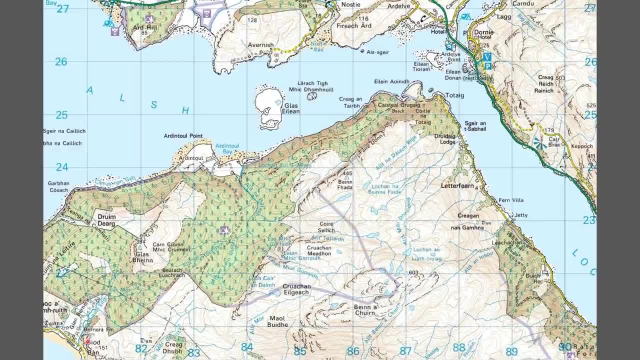 We start from the left-hand side to try and identify the first easting that comes into contact with this square And as we read along we come into contact with it over here: 87. So the first part of the four-figure grid reference would be 87.. 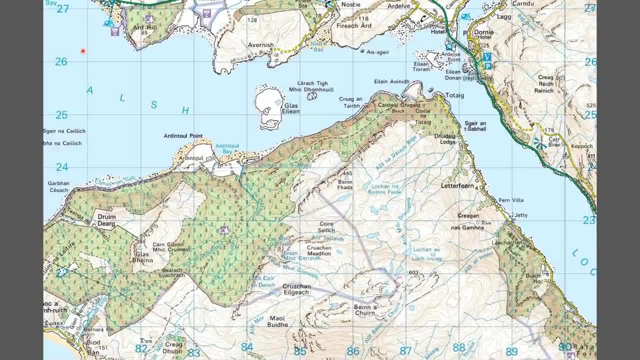 Then we start reading the northings. The northing that comes into contact over here is 26.. So the grid reference for this square is 8726.. And if we want to be more precise and we want to find this parking over here, 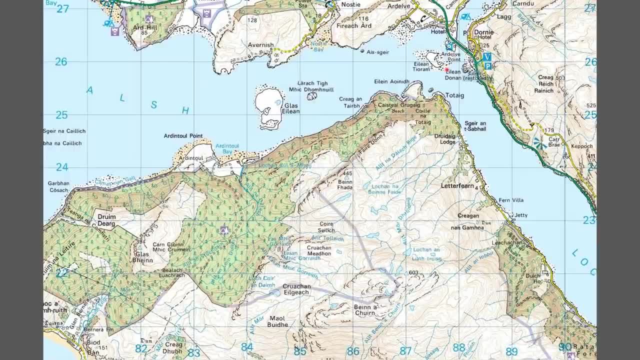 we can see that it's 87, probably 878,, this point here, 26, and I would say 3.. So 878, 263.. Now, sometimes on a grid reference, you have to be a little bit careful about symbols. 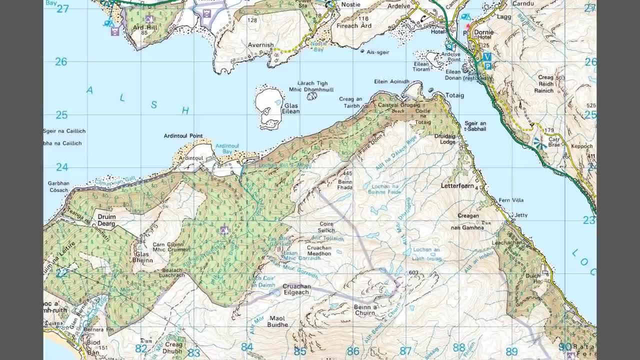 There's an excellent one over here. Do we see this caravan and camping site? Now the symbol is actually at grid reference 881269 or 268.. But that's not the grid reference of where this is found in real life. Do we see this little line that's coming from it? 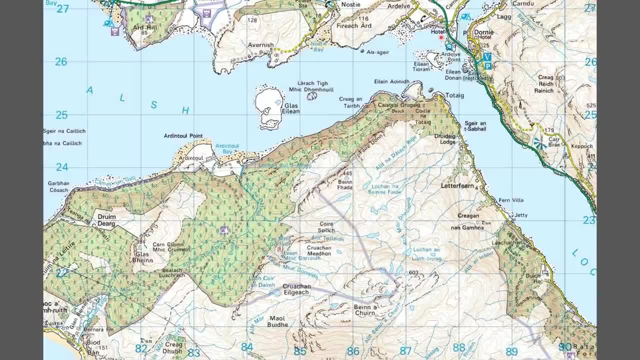 This is trying to indicate exactly where it's found. Sometimes in ordinate survey maps you can't fit the symbols into the right area, otherwise it gets too crowded, So they will put them off in a spare bit of the map, like this one, and then connect it with an arrow. 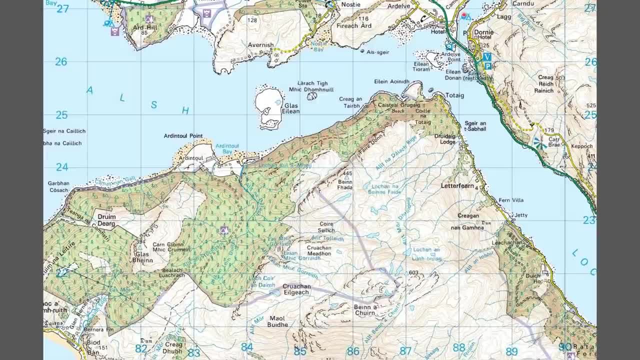 So be very careful about that. So the caravan and campsite that you can see over here is actually not found in the four-figure grid reference 8826, but it's found exactly over here where my laser pointer is looking at now. You can see a similar situation with this telephone box over here.